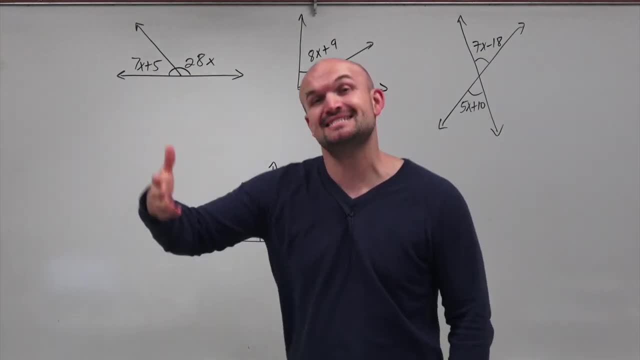 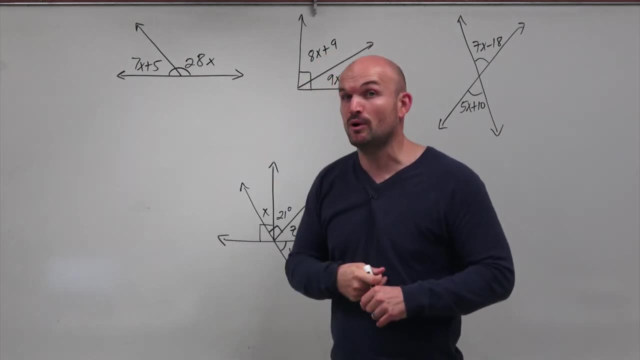 angles that make up a line. they are called the linear pair as well as supplementary. Now, what's important about them being supplementary is that we know that the sum of those two angles is going to add up to 180 degrees. So if I need to find the measure of these two angles- or at least 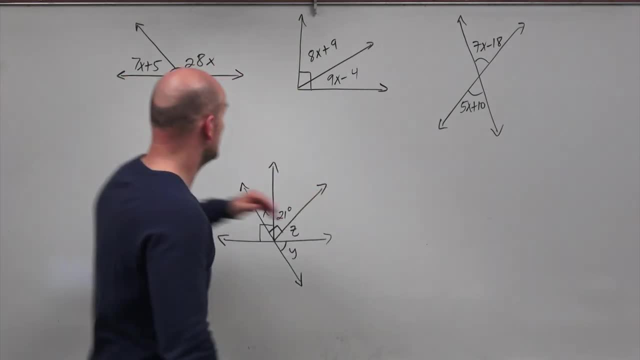 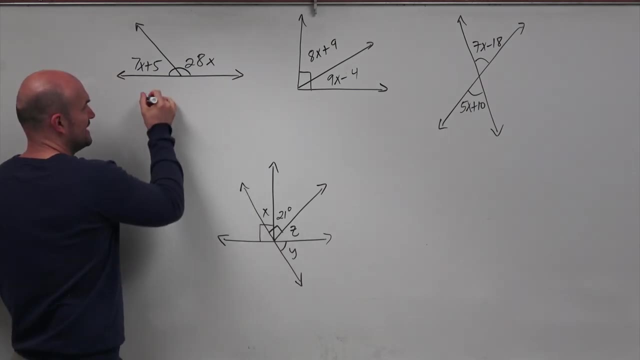 solve for x. what I need to do is create an equation. So, if I know, these two angles are supplementary, a linear pair. therefore supplementary that means they add up to 180 degrees. So I can say: 7x plus 5 plus a 28x equals 180 degrees. Now, if I needed to find the measure, 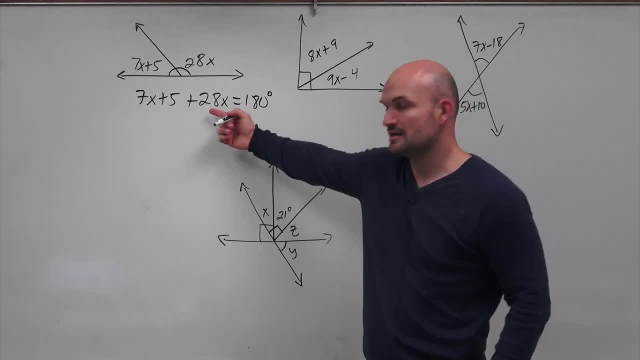 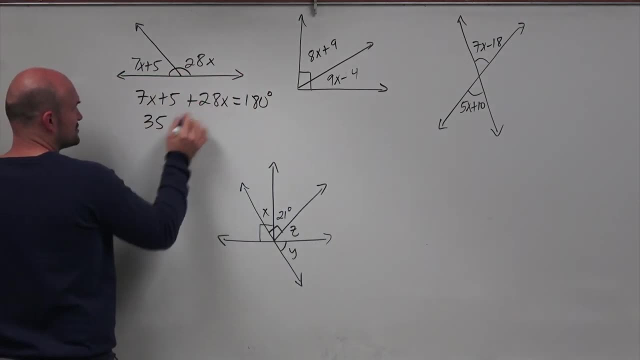 of either one of these angles. all I would simply need to do is solve for x. So on the left-hand side, I need to kind of clean that up a little bit And I combine this to give me: 7x plus 28x is a 35x plus 5 equals 180 degrees. Now I'll just subtract a 5 here And I get a 35x equals. 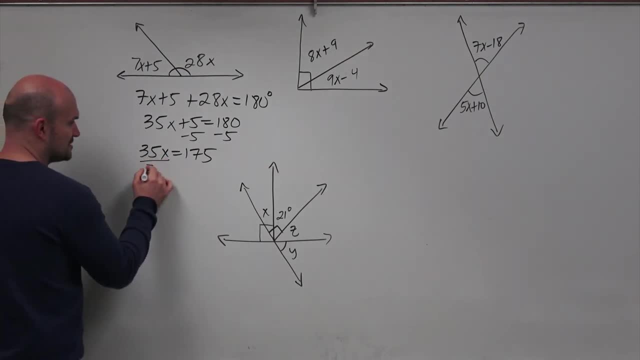 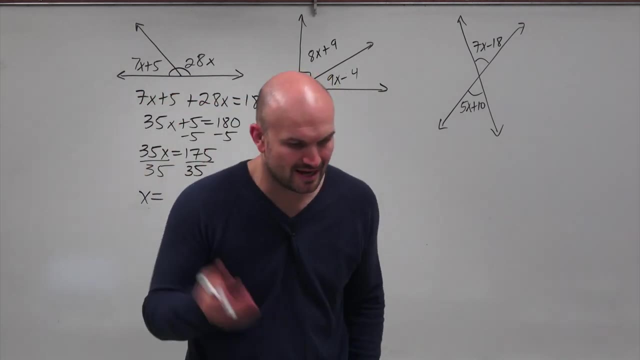 175.. Then to solve for x, I'll just divide by 35 on both sides And I get x equals. well, how many times does x go into 35?? I know, 30 times 5 is 150. And therefore you can see that'd be a. 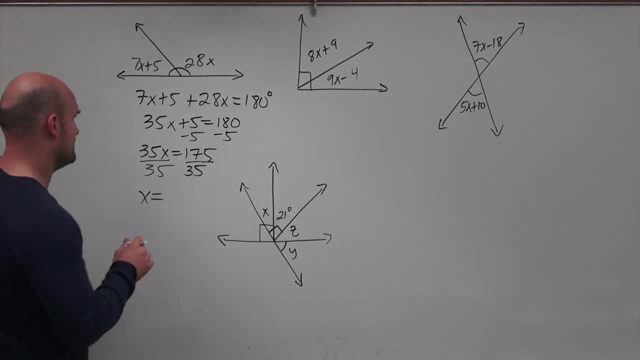 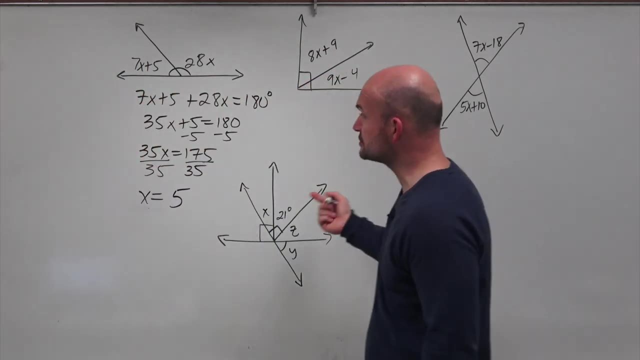 5.. That's going to be an extra. 3 times 5 would be 5.. And then 5 times 5 is 25.. So that's going to be 5 times. Now again, if I needed to be able to figure out what these measures are, all I need to. 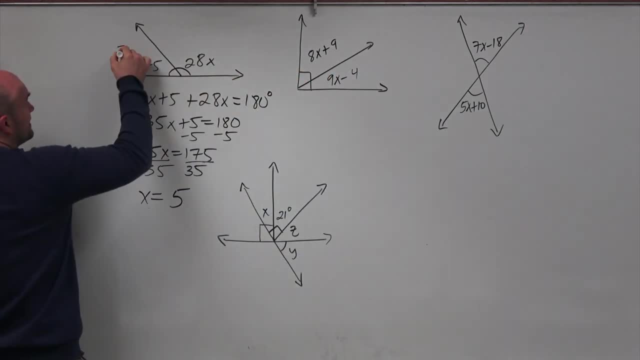 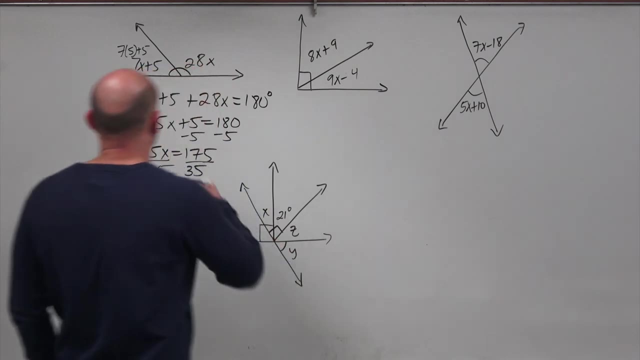 simply do is replace my x with 5.. So I could say 7 times 5 plus 5.. Well, 7 times 5 is going to be 35 plus 5 is 40. So we can say that angle is going to be 40 degrees. And then here you just do 28. 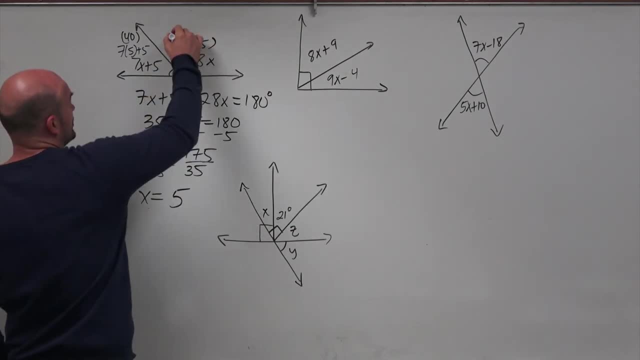 times 5, right, And 28 times 5 is 40. And then here you just do 28 times 5, right, And 28 times 5 is going to be 140 degrees, And you could use degrees or not, depending on what the problem is. 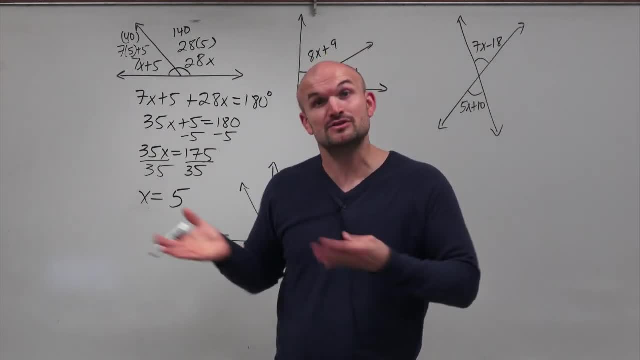 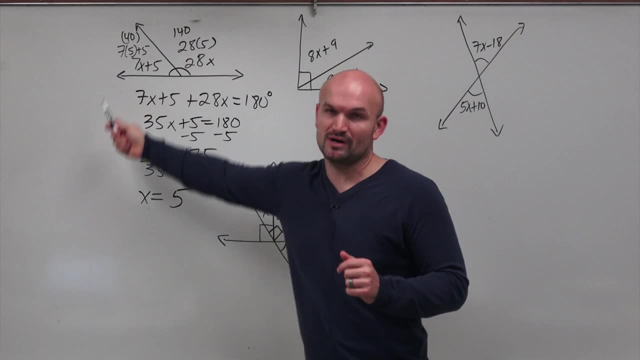 But there we go. That's how you'd use when you have supplementary angles or, in this diagram, represented as a linear pair, Because not all supplementary angles are a linear pair. It's just important if they create a line. The next example: you can see that these create a right angle. 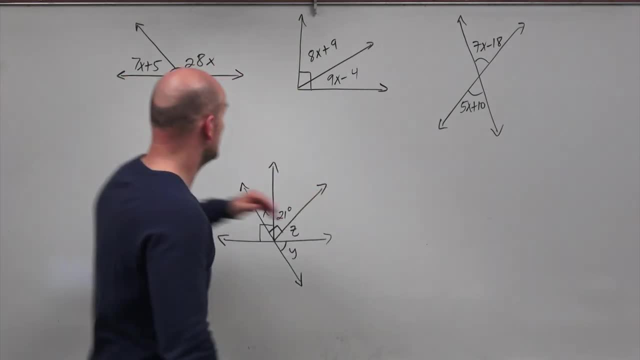 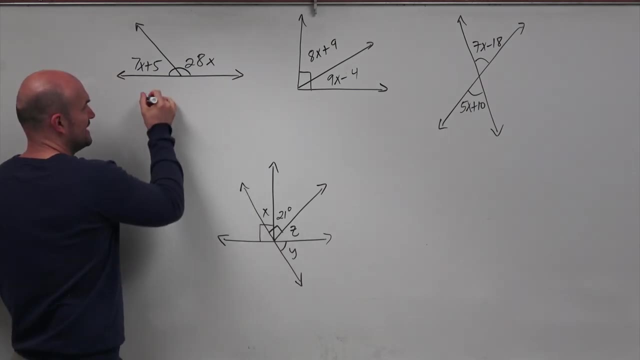 solve for x. what I need to do is create an equation. So, if I know, these two angles are supplementary, a linear pair. therefore supplementary that means they add up to 180 degrees. So I can say: 7x plus 5 plus a 28x equals 180 degrees. Now, if I needed to find the measure, 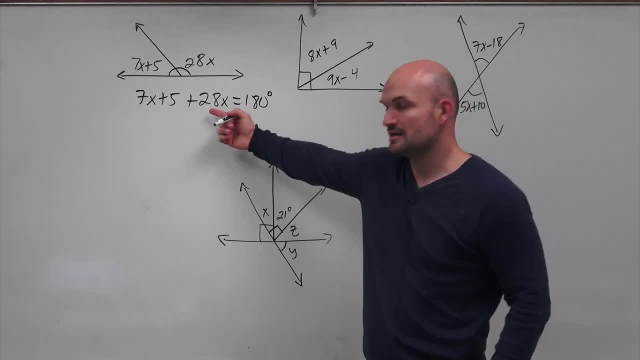 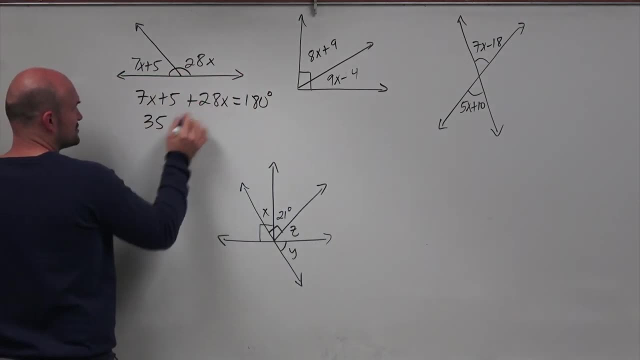 of either one of these angles. all I would simply need to do is solve for x. So on the left-hand side, I need to kind of clean that up a little bit And I combine this to give me: 7x plus 28x is a 35x plus 5 equals 180 degrees. Now I'll just subtract a 5 here And I get a 35x equals. 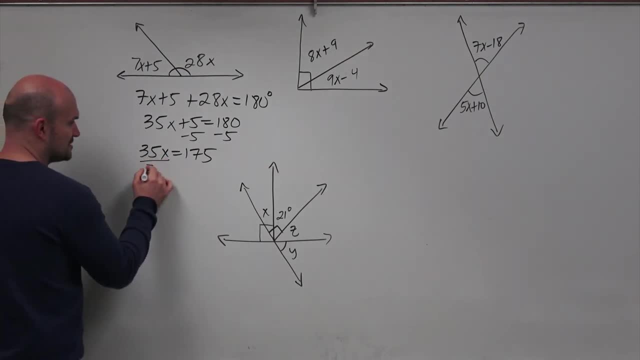 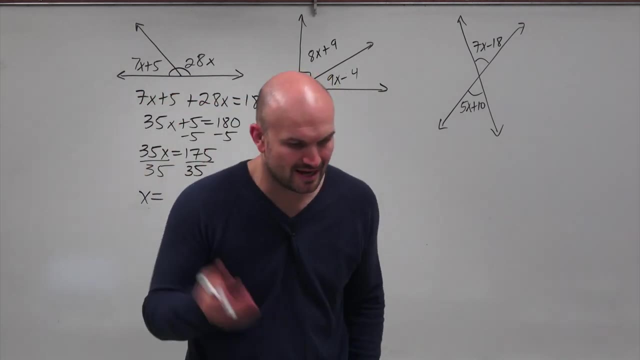 175.. Then to solve for x, I'll just divide by 35 on both sides And I get x equals. well, how many times does x go into 35?? I know, 30 times 5 is 150. And therefore you can see that'd be a. 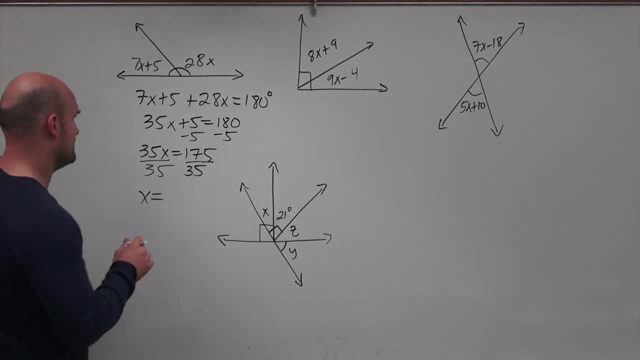 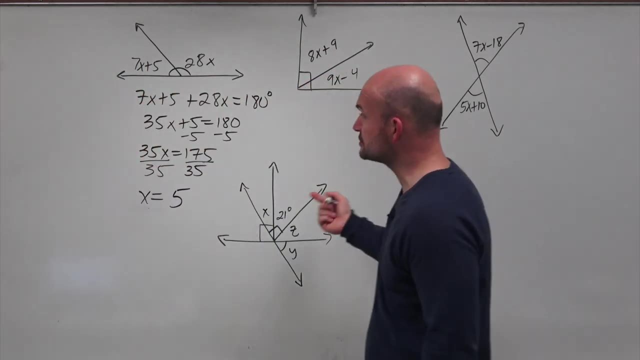 5.. That's going to be an extra. 3 times 5 would be 5.. And then 5 times 5 is 25.. So that's going to be 5 times. Now again, if I needed to be able to figure out what these measures are, all I need to. 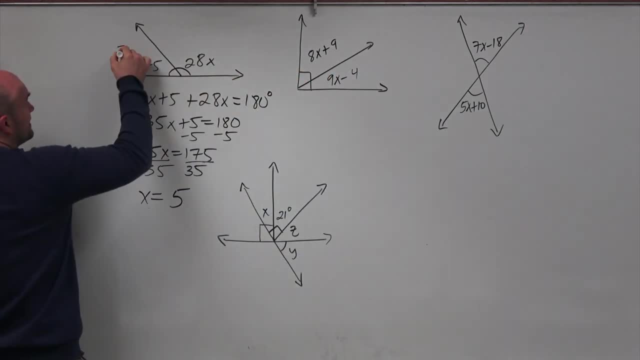 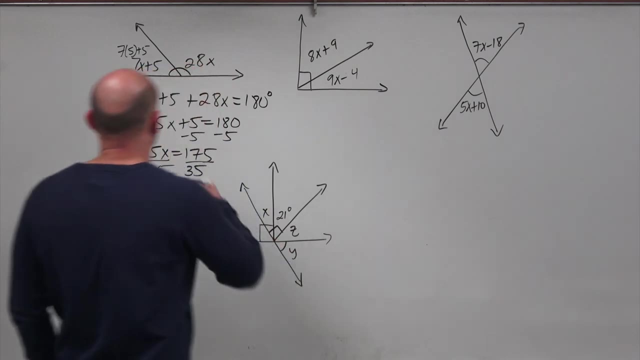 simply do is replace my x with 5.. So I could say 7 times 5 plus 5.. Well, 7 times 5 is going to be 35 plus 5 is 40. So we can say that angle is going to be 40 degrees. And then here you just do 28. 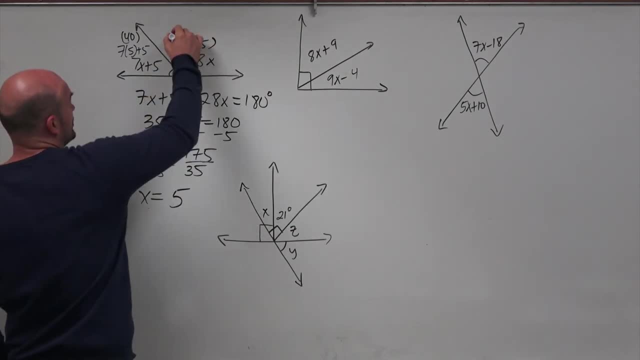 times 5, right, And 28 times 5 is 40. And then here you just do 28 times 5, right, And 28 times 5 is going to be 140 degrees, And you could use degrees or not, depending on what the problem is. 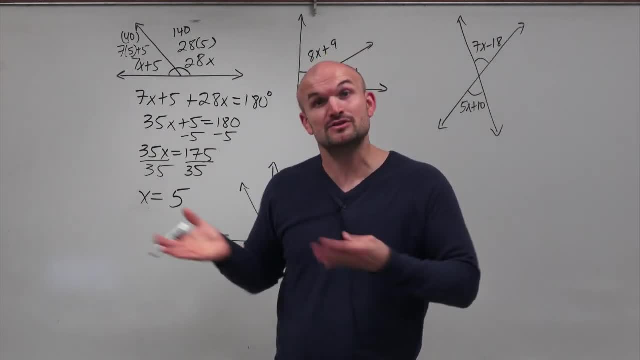 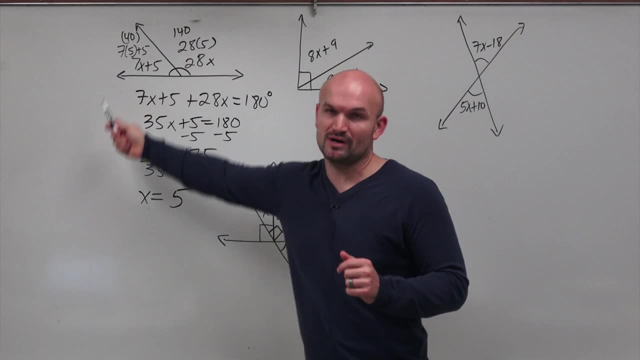 But there we go. That's how you'd use when you have supplementary angles or, in this diagram, represented as a linear pair, Because not all supplementary angles are a linear pair. It's just important if they create a line. The next example: you can see that these create a right angle. 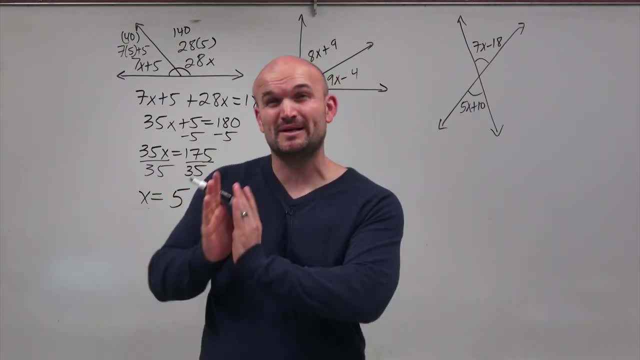 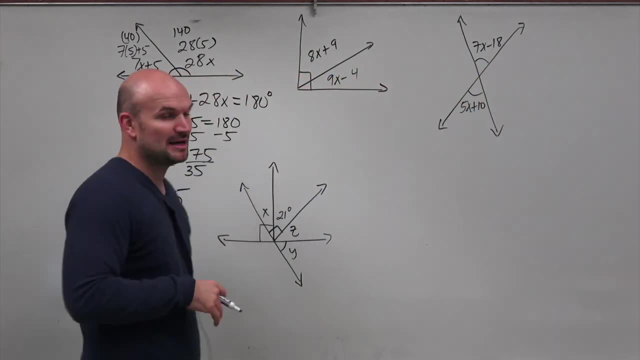 right, And any two times you have two angles that add up to create a right angle. we call them complementary angles, So again the relationship just kind of like supplementary. the sum of two angles that are complementary is 90 degrees, So again I could write another. 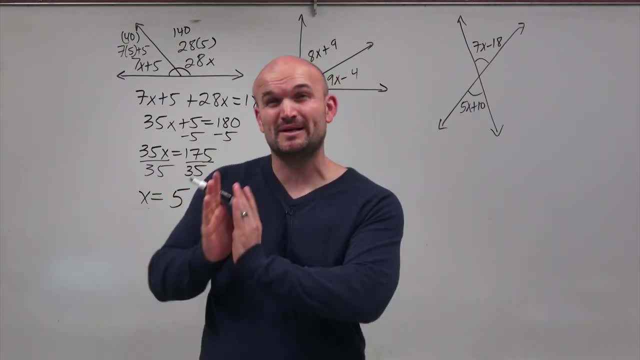 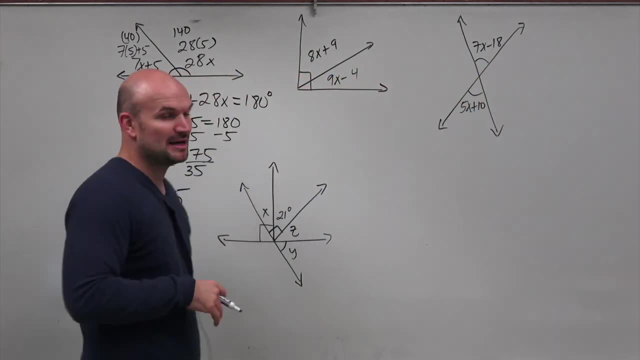 right, And any two times you have two angles that add up to create a right angle. we call them complementary angles, So again the relationship just kind of like supplementary. the sum of two angles that are complementary is 90 degrees, So again I could write another. 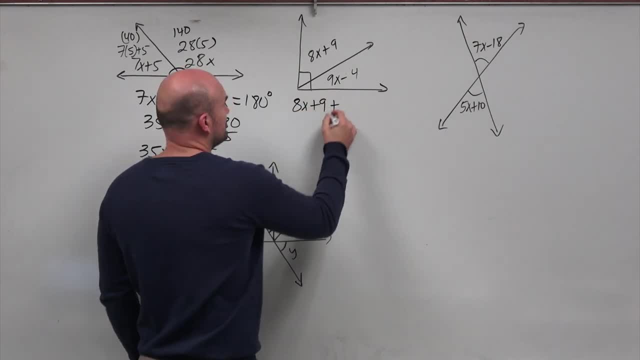 equation I can say an 8x plus 9 plus 9x minus 4.. These don't add to 180 like our linear pair. These add to 90 degrees. So again now, all I need to do to solve for x before I can identify the. 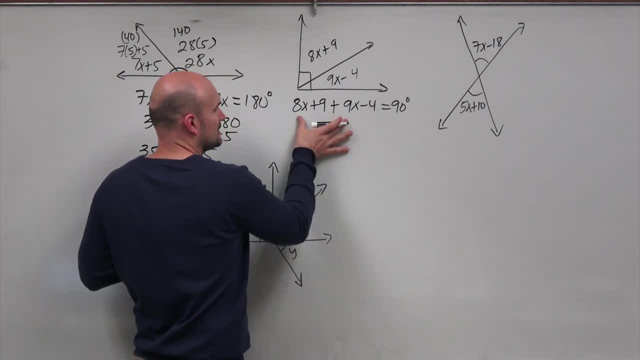 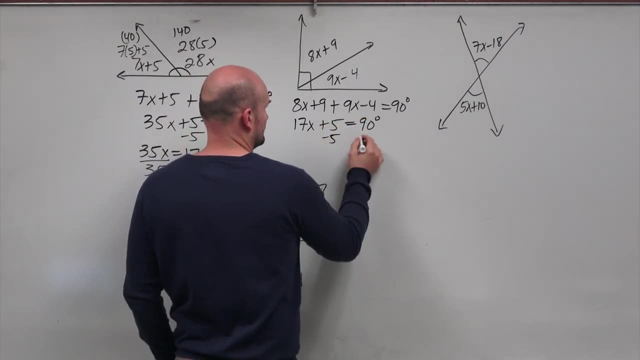 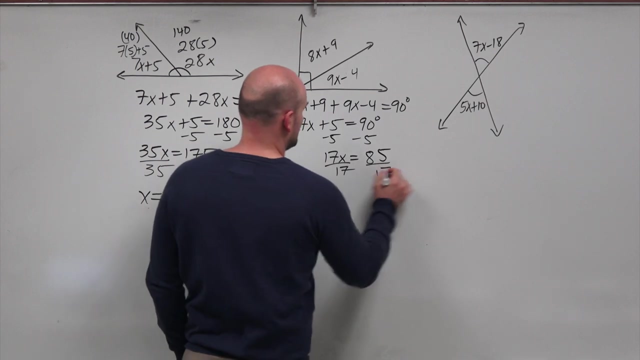 value of these two angles here is: I can clean these up here and give me a 17x And let's see: plus 5 equals A 90 degrees Subtract 5, and I get 17x equals 85. And then divide by 17, here And again. 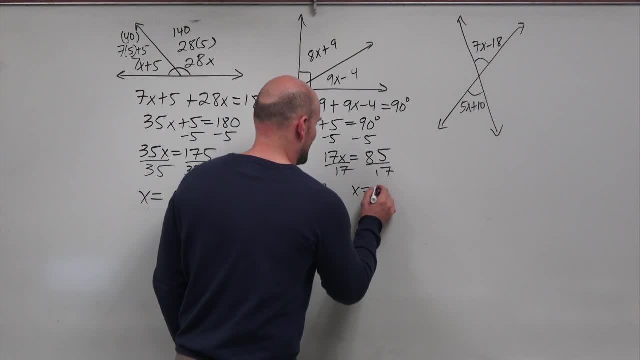 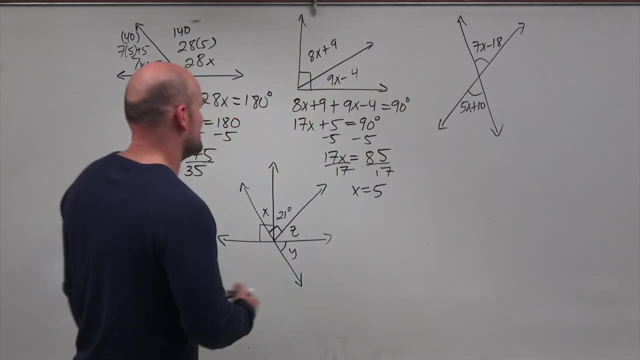 it looks like you're going to get a 50.. That'd be 35. So x is equal to 5.. And I didn't mean for these all to equal 5.. But you could again kind of rework this the exact same way. Take my 5 and. 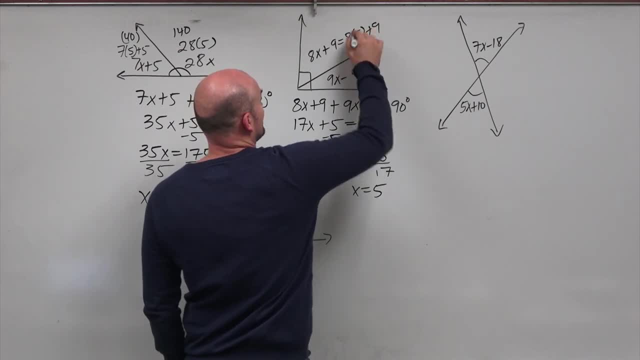 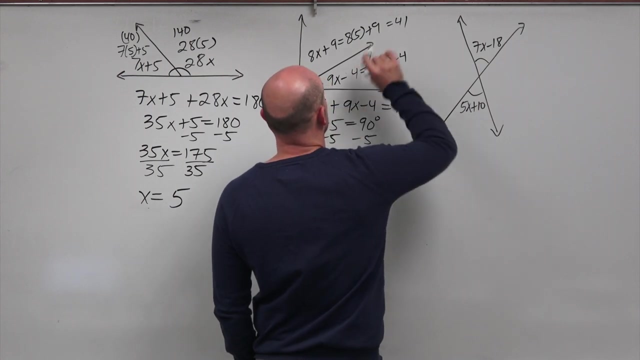 plug it in, So I have an 8 times 5 plus 9.. 8 times 5 is 40, plus 9 is 41. And then here I can do 9 times 5 minus 4.. 9 times 5 is 45, minus 4 is 40. That's a 49, sorry, And that's. 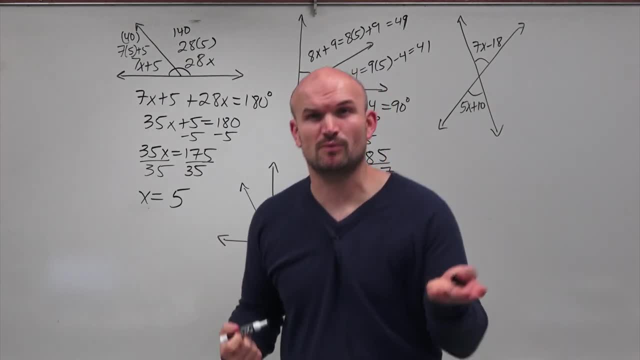 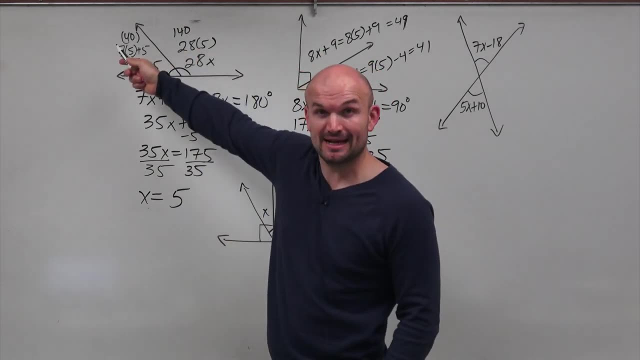 41.. Now again, one thing I forgot to mention is you can always check your work Again. I said: two angles that are supplementary add up to 180.. Does 140 and 40, does that add up to 180?? It does. 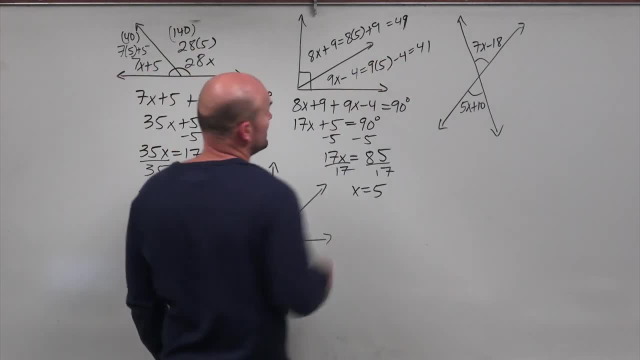 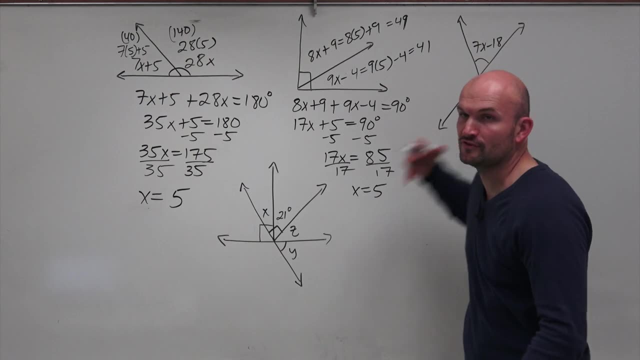 Right. What about 49 and 41?? Does that add up to 90?? And yes, it does. All right, Now the last angle relationship we're going to investigate in this video is our vertical angles. Vertical angles are two angles that share a common vertex but do not share a common side. 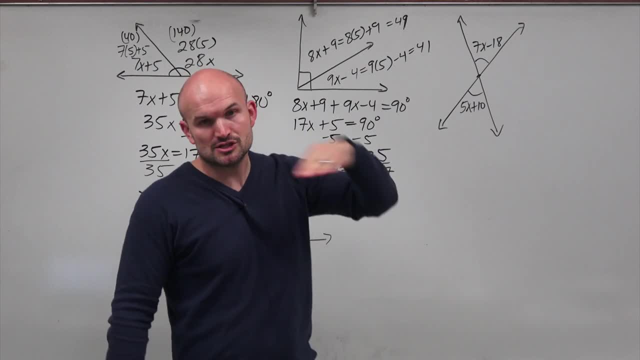 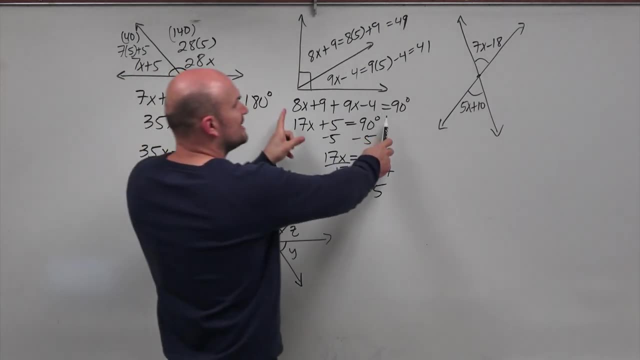 So you can see these do not have too many sides, but they do have a common vertex. So vertical angles are created when you have intersecting lines, And vertical angles- unlike supplementary angles, unlike complementary angles- are going to be equal to one another. So the equation that 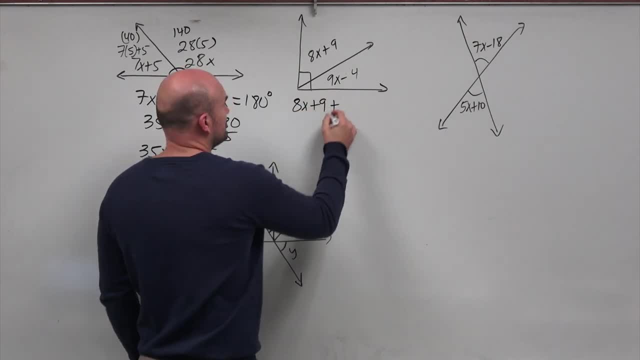 equation I can say an 8x plus 9 plus 9x minus 4.. These don't add to 180 like our linear pair. These add to 90 degrees. So again now, all I need to do to solve for x before I can identify the. 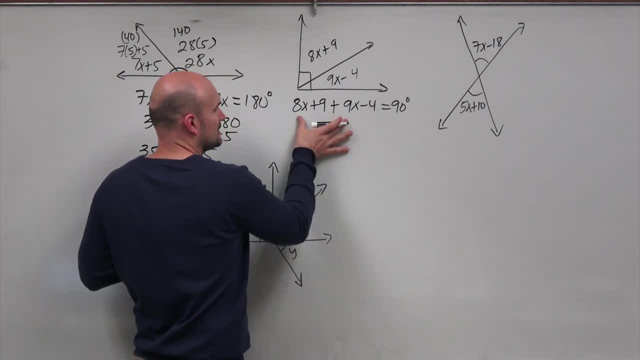 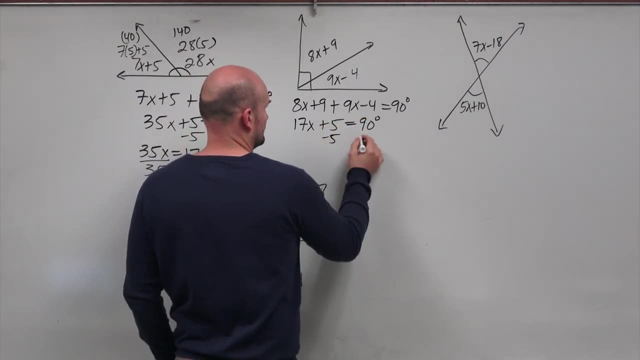 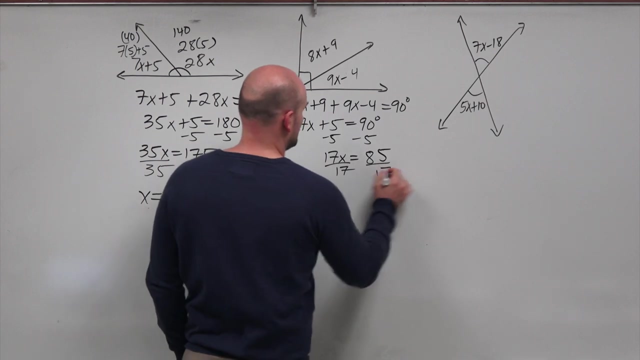 value of these two angles here is: I can clean these up here and give me a 17x And let's see: plus 5 equals A 90 degrees Subtract 5, and I get 17x equals 85. And then divide by 17, here And again. 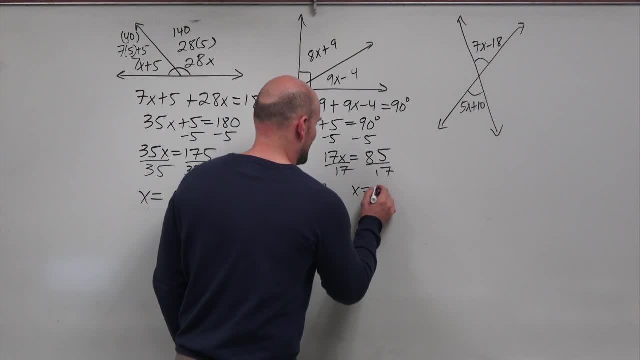 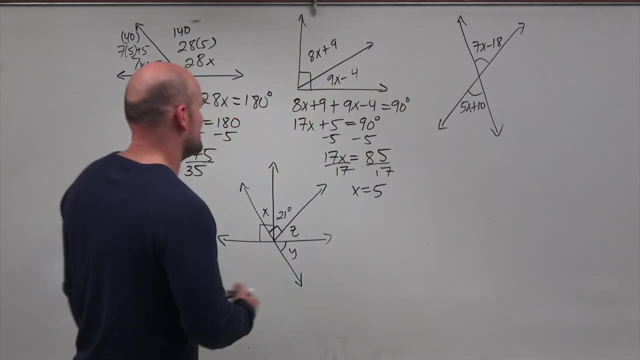 it looks like you're going to get a 50.. That'd be 35. So x is equal to 5.. And I didn't mean for these all to equal 5.. But you could again kind of rework this the exact same way. Take my 5 and. 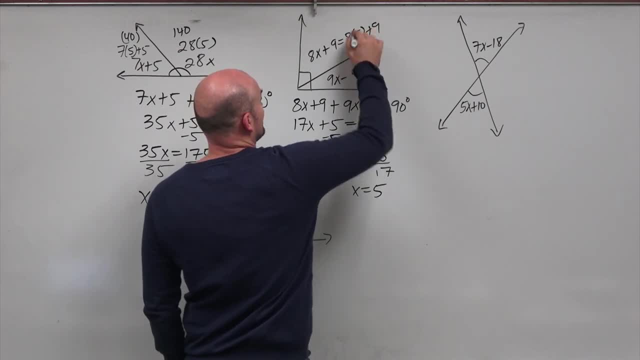 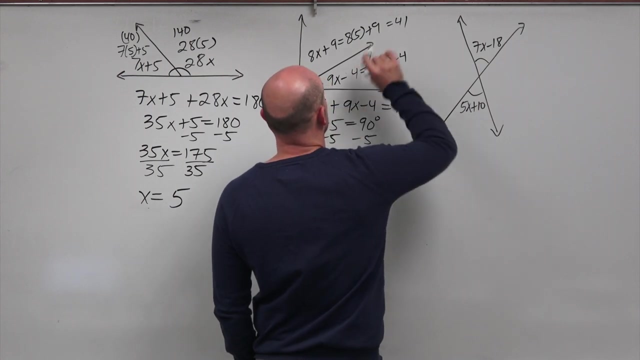 plug it in, So I have an 8 times 5 plus 9.. 8 times 5 is 40, plus 9 is 41. And then here I can do 9 times 5 minus 4.. 9 times 5 is 45, minus 4 is 40. That's a 49, sorry, And that's. 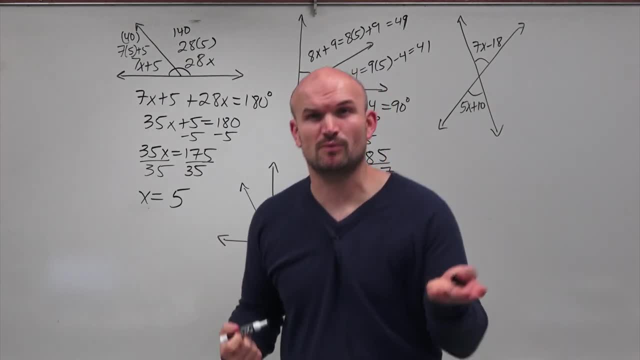 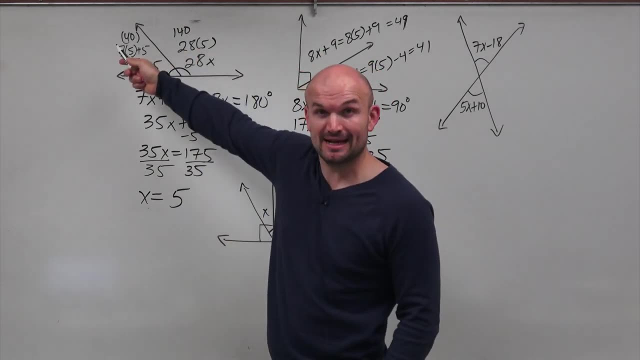 41.. Now again, one thing I forgot to mention is you can always check your work Again. I said: two angles that are supplementary add up to 180.. Does 140 and 40, does that add up to 180?? It does. 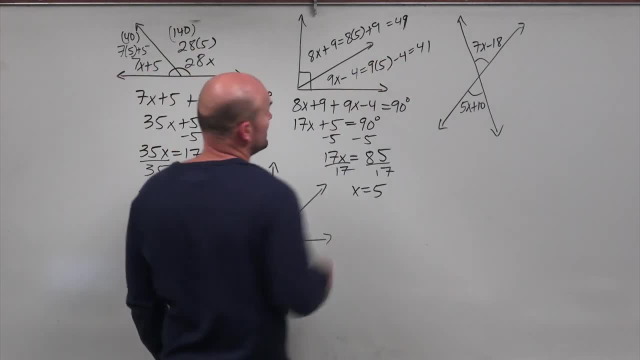 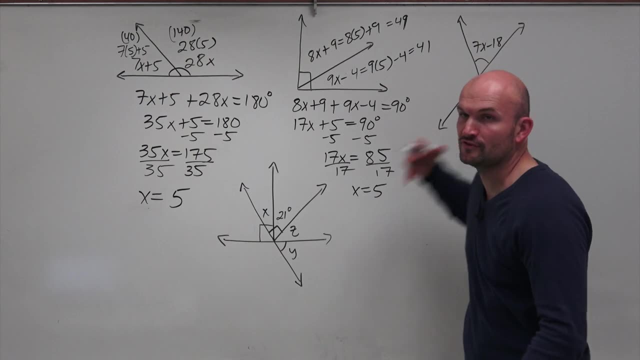 Right. What about 49 and 41?? Does that add up to 90?? And yes, it does. All right, Now the last angle relationship we're going to investigate in this video is our vertical angles. Vertical angles are two angles that share a common vertex but do not share a common side. 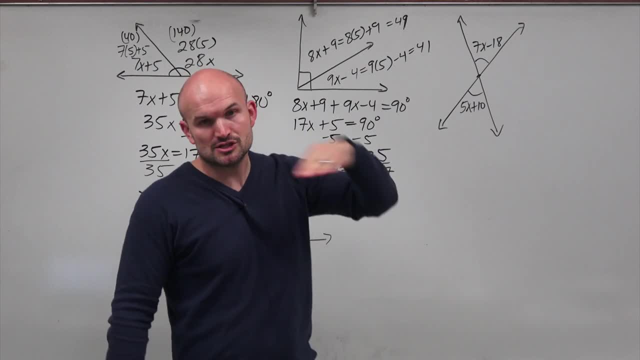 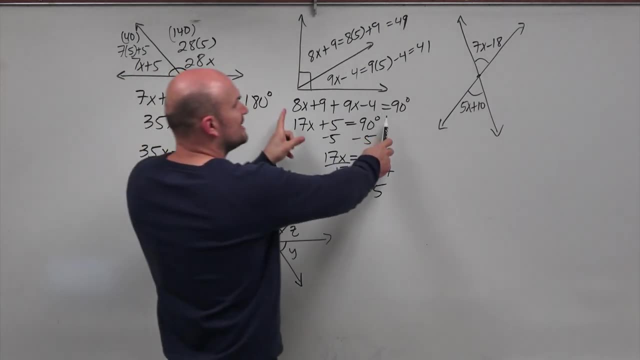 So you can see these do not have too many sides, but they do have a common vertex. So vertical angles are created when you have intersecting lines, And vertical angles- unlike supplementary angles, unlike complementary angles- are going to be equal to one another. So the equation that 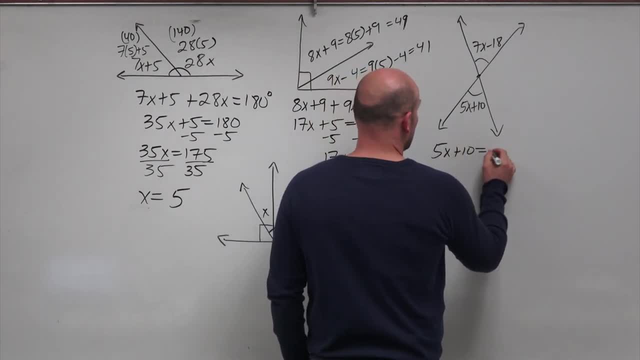 I'm going to write here to find these values is 5x plus 10 equals 7x plus 10.. So I'm going to have an x minus 18.. So now I have a variable on both sides To solve a problem like this. I'm 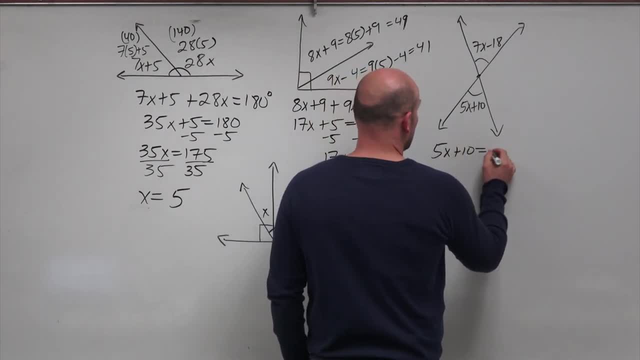 I'm going to write here to find these values is 5x plus 10 equals 7x plus 10.. So I'm going to have an x minus 18.. So now I have a variable on both sides To solve a problem like this. I'm 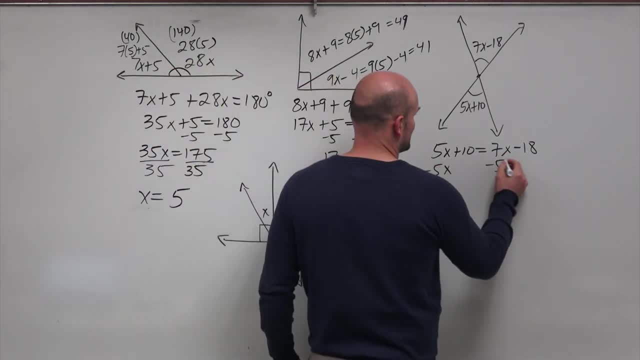 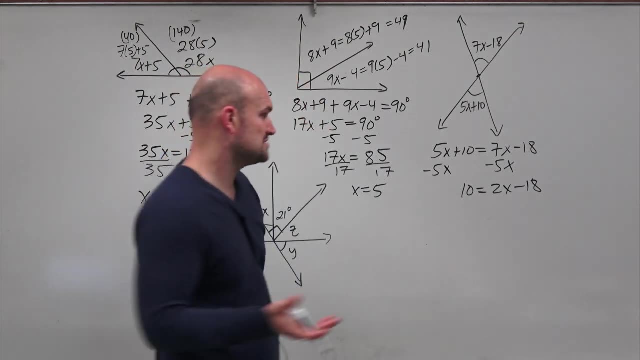 going to need to get the variable to the same side. So I'm going to subtract the 5x here on both sides. Then we give me a 10 equals 2x minus 18.. And now I have a two-step equation that I can. 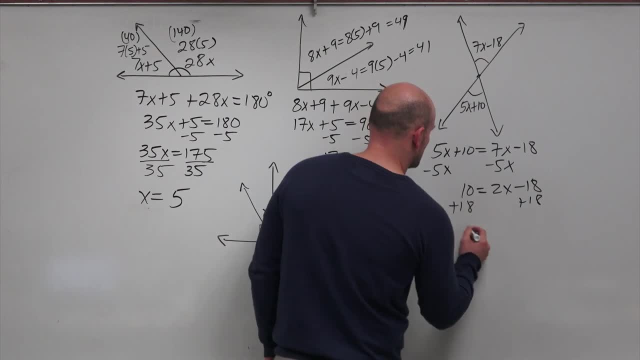 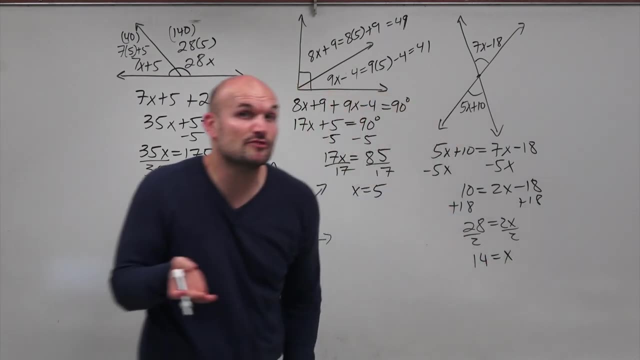 go ahead and solve for. So I'll add the 18 to both sides And I get 28 equals 2x divided by 2, divided by 2.. 14 equals x. Now the cool thing about vertical angles is, since they're equal to. 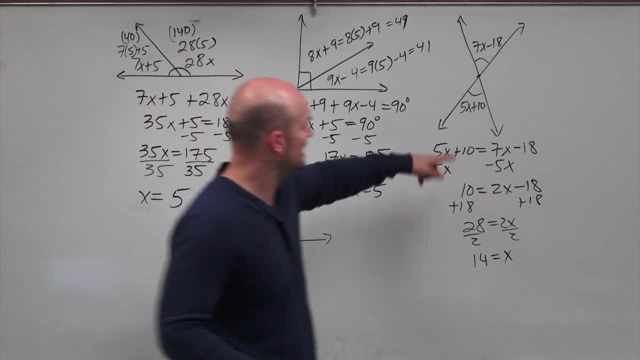 one another. all I simply need to do is find the measure of one of those angles, And I know that's going to be the measure of the other one. So again, we found the value of x. So now let's find the value of. 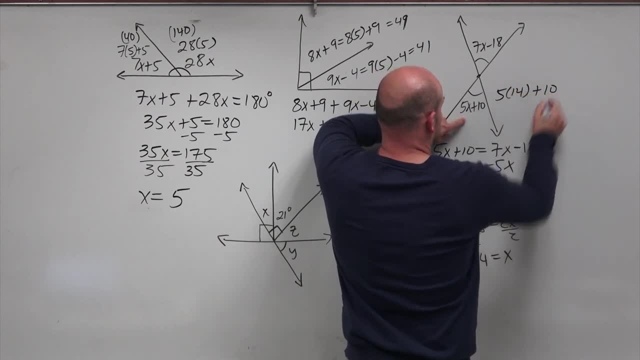 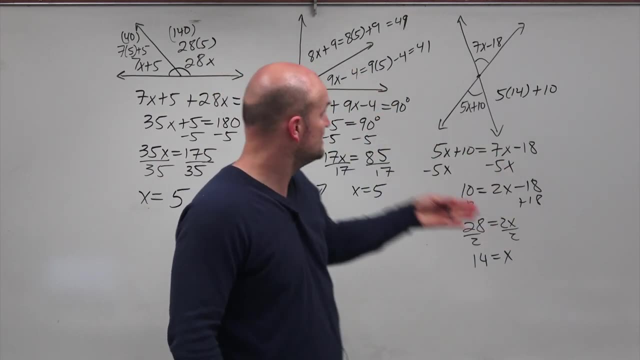 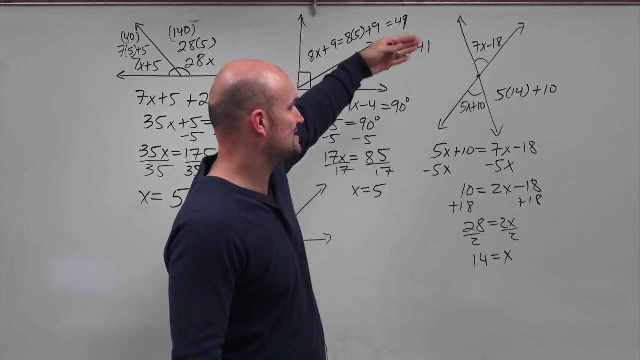 this angle. So I'll do 5 times 14 plus 10.. Well, 14 times 2 is 28.. Times 4 is going to be 56. And therefore that would be a 70.. Or 5 times 10 is 50.. Times 5 times 4 is 20.. So that's 70 plus. 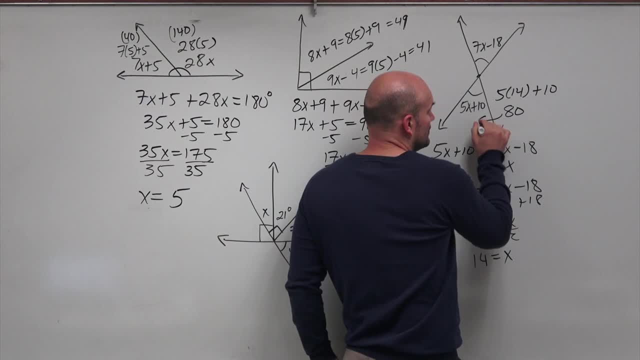 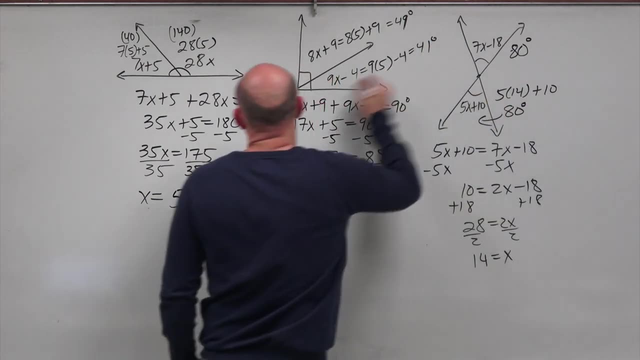 10 is going to be 80. So if this is 80, then I know that that also has to be 80. And again, these are all going to be degrees. I guess I should probably not be as lazy and give you a nice little degree symbol for each of those. Now, how are we? 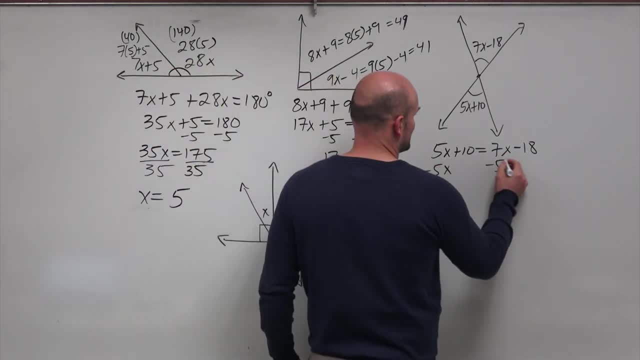 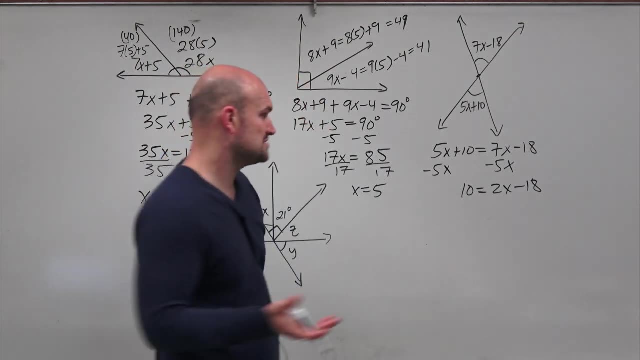 going to need to get the variable to the same side. So I'm going to subtract the 5x here on both sides. Then we give me a 10 equals 2x minus 18.. And now I have a two-step equation that I can. 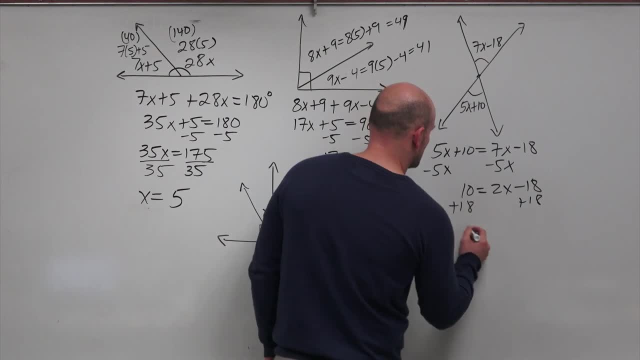 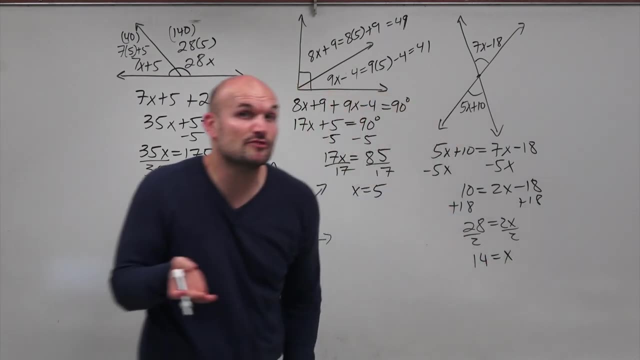 go ahead and solve for. So I'll add the 18 to both sides And I get 28 equals 2x divided by 2, divided by 2.. 14 equals x. Now the cool thing about vertical angles is, since they're equal to. 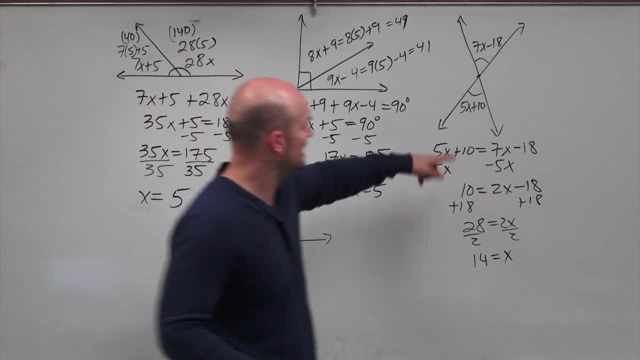 one another. all I simply need to do is find the measure of one of those angles, And I know that's going to be the measure of the other one. So again, we found the value of x. So now let's find the value of. 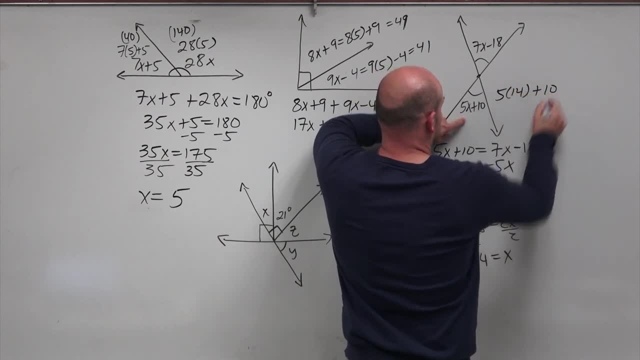 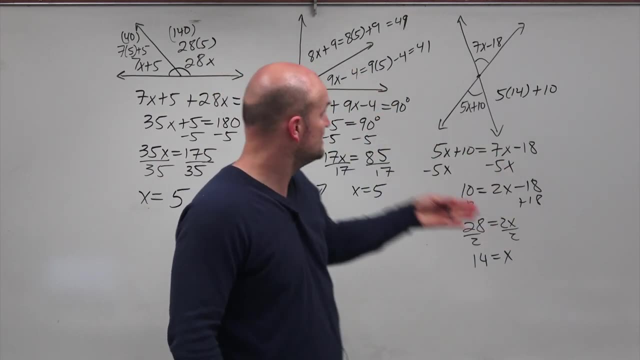 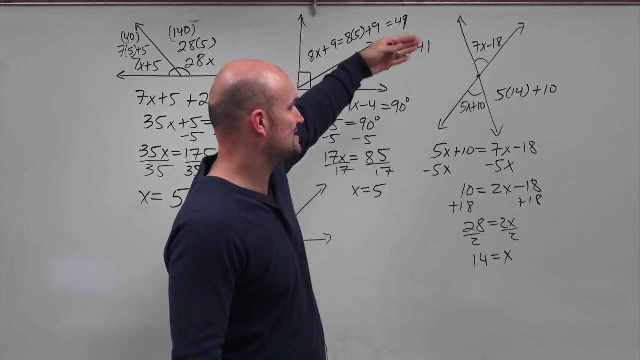 this angle. So I'll do 5 times 14 plus 10.. Well, 14 times 2 is 28.. Times 4 is going to be 56. And therefore that would be a 70.. Or 5 times 10 is 50.. Times 5 times 4 is 20.. So that's 70 plus. 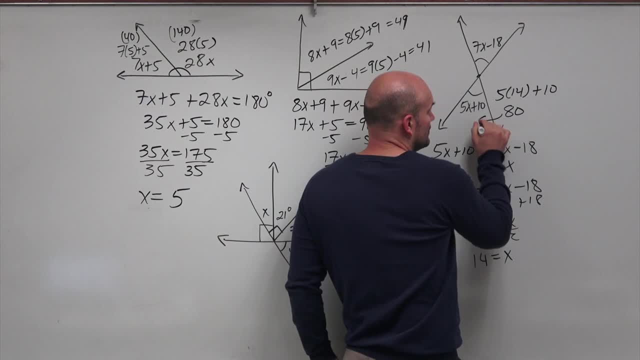 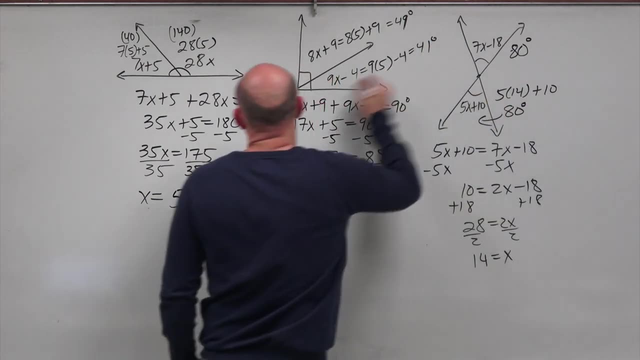 10 is going to be 80. So if this is 80, then I know that that also has to be 80. And again, these are all going to be degrees. I guess I should probably not be as lazy and give you a nice little degree symbol for each of those. Now, how are we? 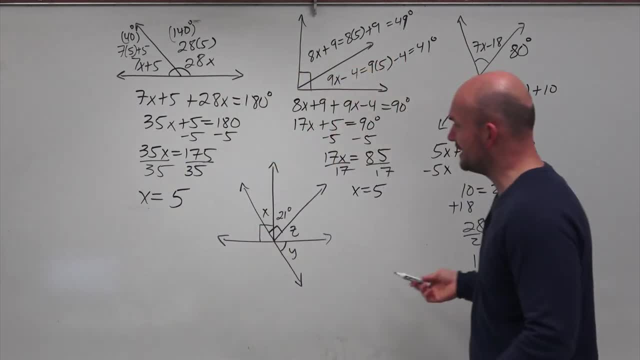 going to use all of this. How can we use all this information now to solve a figure like this? So I'm getting rid of the. Now I have not just one variable, but I have an x, y and z, And you can. 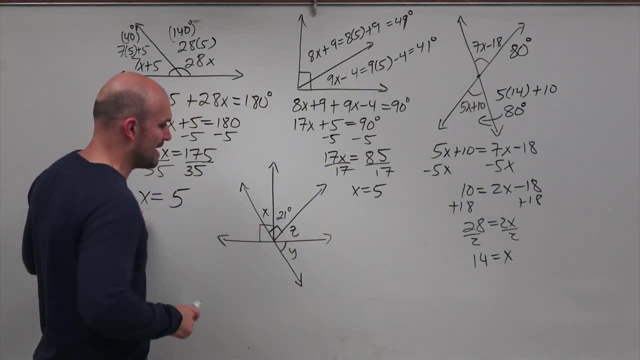 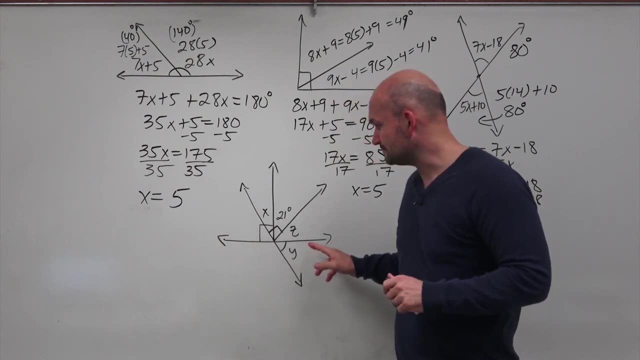 see all of these angle relationships are being represented on one graph. So the first thing I recognize is: I see that little box And I remember that box represents that all of these angles are going to be 90 degrees. I'm sorry, These two angles are going to add to give me a 90 degrees. So how? 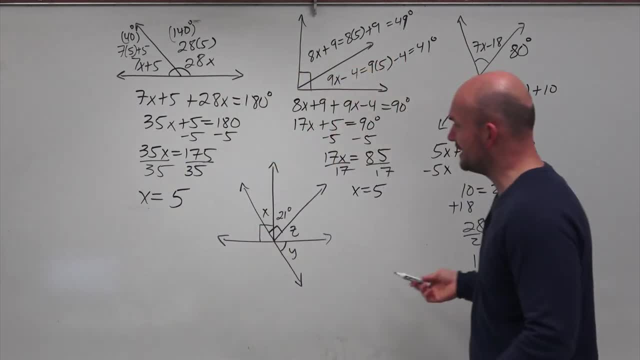 going to use all of this. How can we use all this information now to solve a figure like this? So I'm getting rid of the. Now I have not just one variable, but I have an x, y and z, And you can. 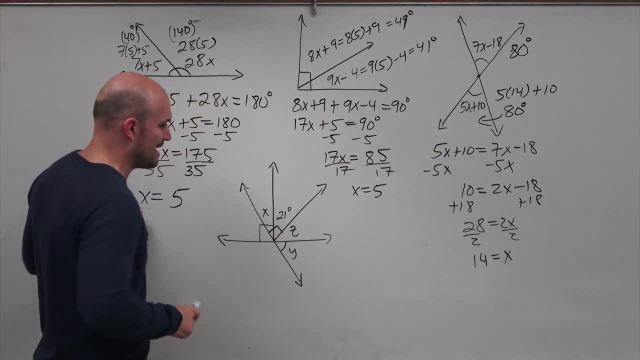 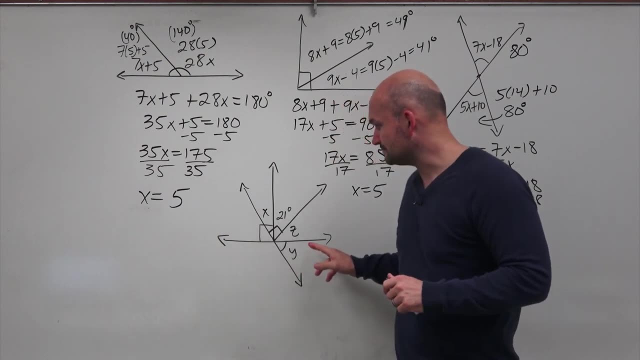 see all of these angle relationships are being represented on one graph. So the first thing I recognize is: I see that little box And I remember that box represents that all of these angles are going to be 90 degrees. I'm sorry, These two angles are going to add to give me a 90 degrees. So how? 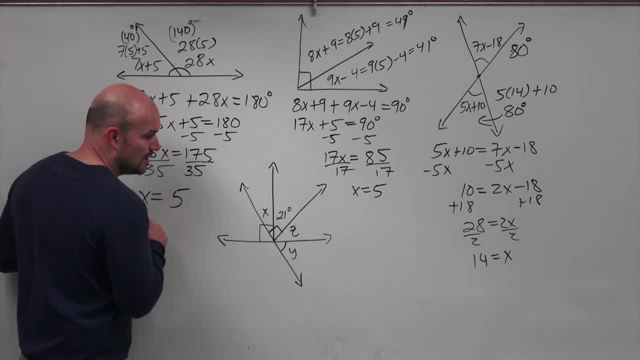 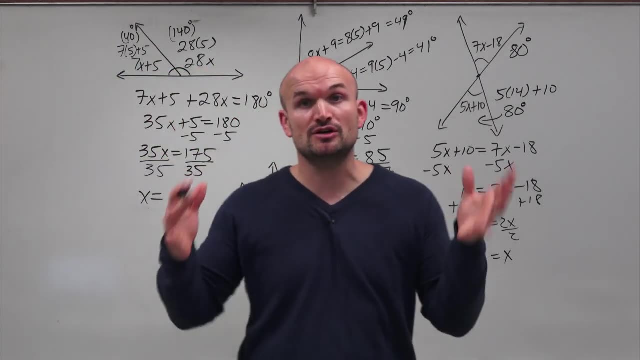 are we going to use all of this information now to solve a figure that looks like this, where I'm going to have not just one variable x, but I have an x, a y and a z. So what we're going to do in this case is look for our 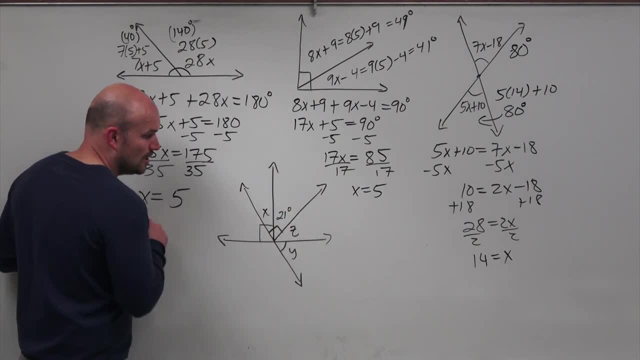 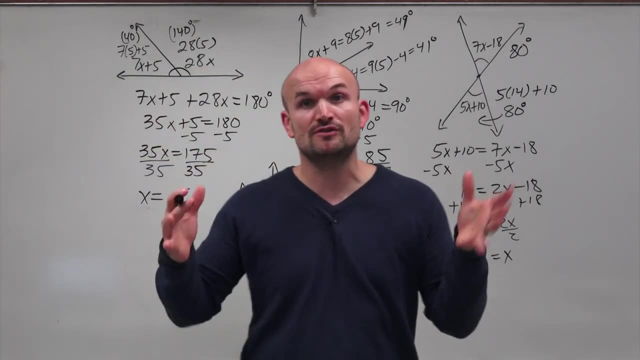 are we going to use all of this information now to solve a figure that looks like this, where I'm going to have not just one variable x, but I have an x, a y and a z. So what we're going to do in this case is look for our 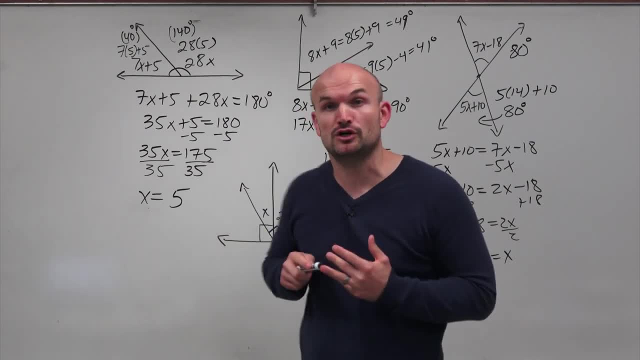 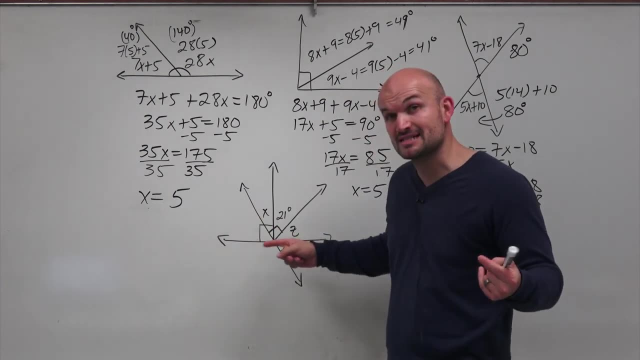 relationships of complementary, supplementary as well as vertical angles. All right, And you can see that I kind of have everything. I have a line right So I can look for supplementary angles. I have these little boxes which represent a 90 degrees And you can see I have some intersecting lines, So I'm going to have 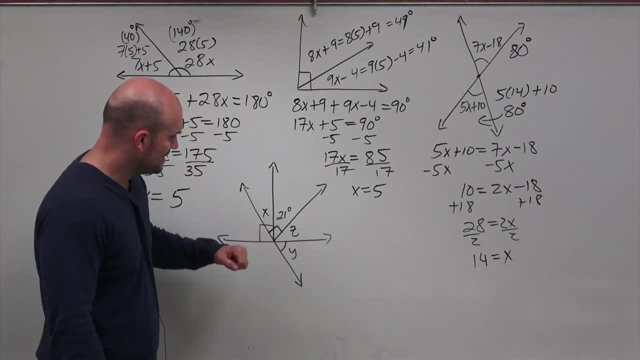 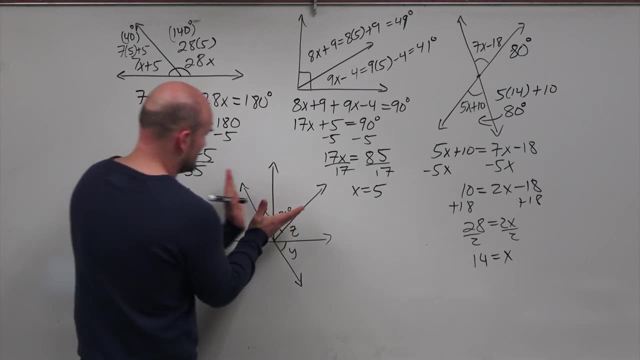 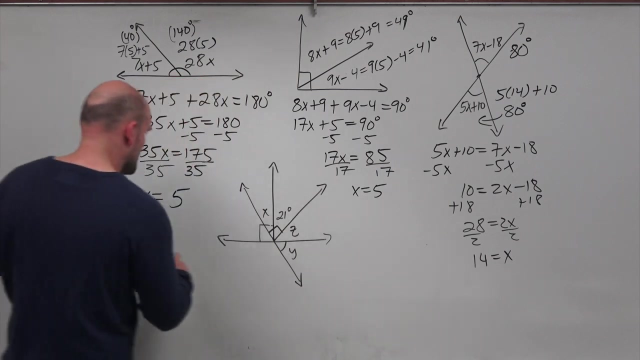 vertical angles. Now, the only angle I have here is 21 degrees And I see that, though, this angle creates a 90-degree angle with this angle x right. So you can see, here is this 90-degree angle. So I know, if this is 21 degrees, then this is going to be the complement of that angle. So I 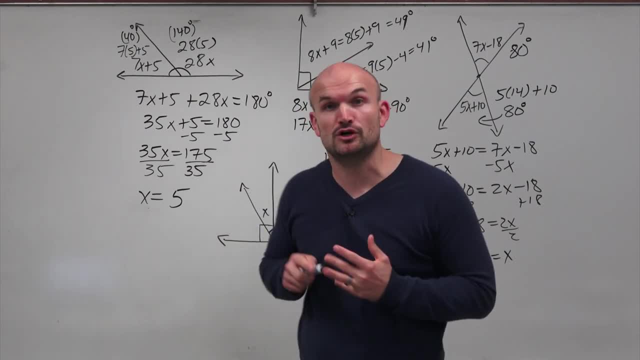 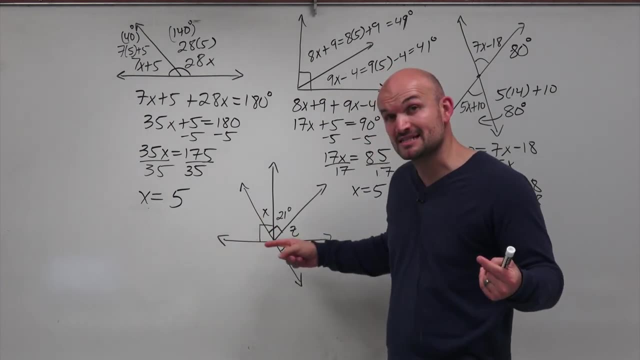 relationships of complementary, supplementary as well as vertical angles. All right, And you can see that I kind of have everything. I have a line right So I can look for supplementary angles. I have these little boxes which represent a 90 degrees And you can see I have some intersecting lines, So I'm going to have 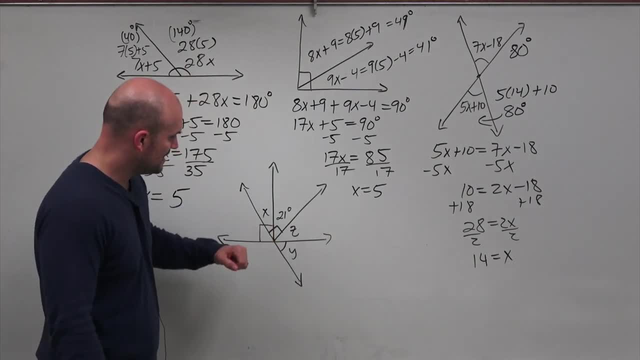 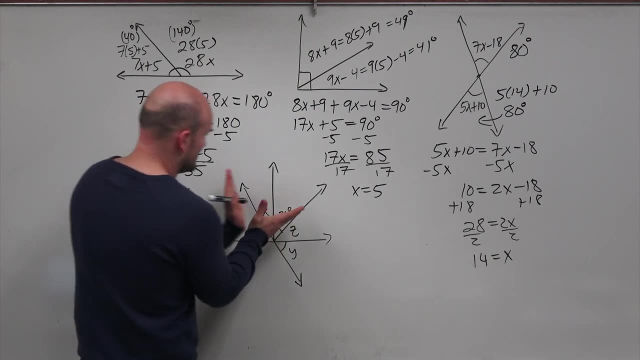 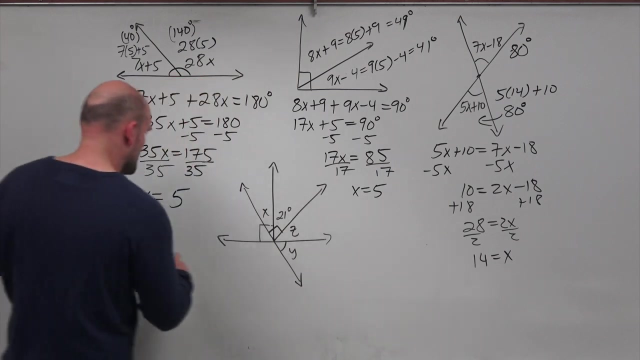 vertical angles. Now, the only angle I have here is 21 degrees And I see that, though, this angle creates a 90 degree angle with this angle x right. So you can see, here is this 90 degree angle. So I know, if this is 21 degrees, then this is going to be the complement of that angle, So I can. 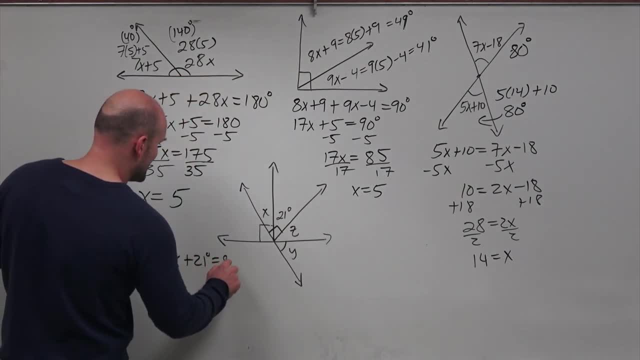 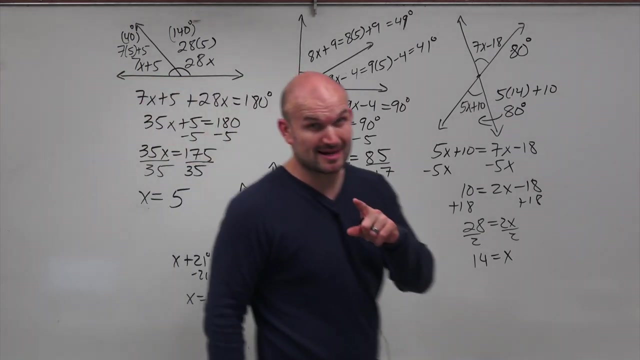 immediately just say: x plus 21 degrees equals 90 degrees. Those are complementary angles. And when I look at 21, I get x equals 69 degrees. So I'm going to write a 69 degrees in here, OK. Now another thing I recognize is 69 degrees, and this angle- whatever this angle is- is also going. 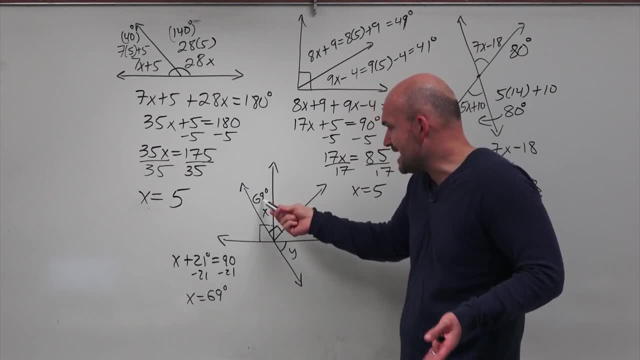 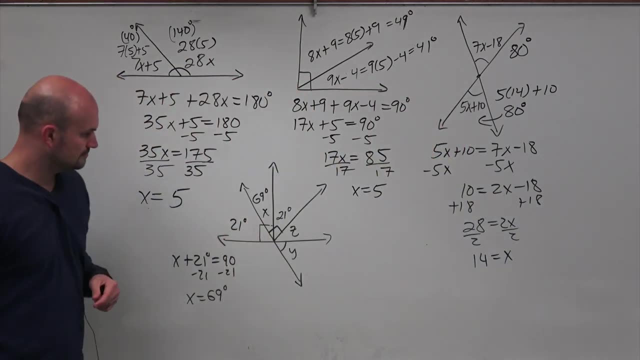 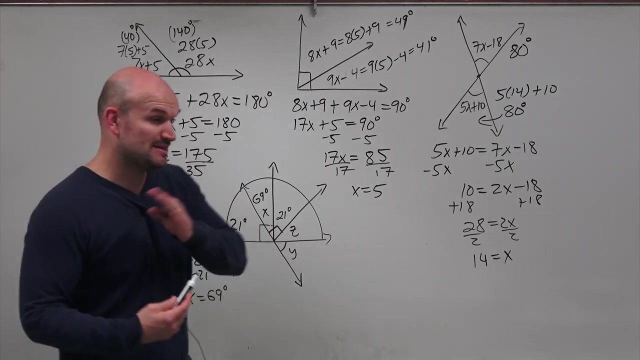 to be complementary, right? And so obviously, if 69 and 21 are complementary, then 69. this has to be 21 degrees as well, OK, So now I want you to look at something. Now, if you look at this, I have this line right. So that means all of these angles are going to add. 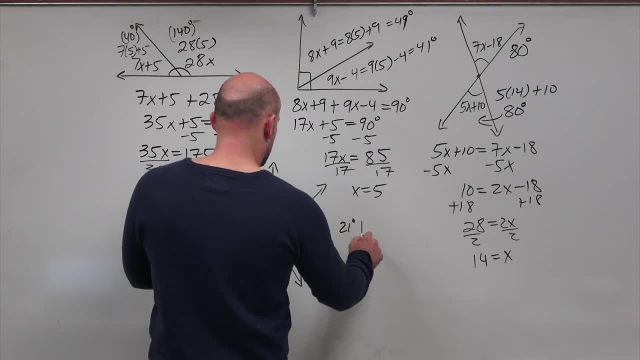 up to 180 degrees. So right now I have 21 degrees plus 69 degrees, plus 21 degrees again plus z. Uh-oh, I'm running out of space. So I have 21 degrees plus 69 degrees, plus 21 degrees plus z. 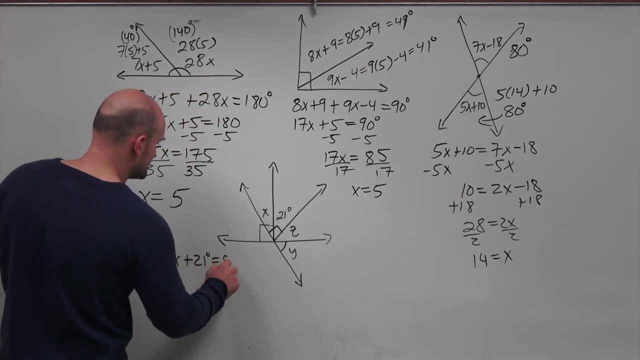 can immediately just say: x plus 21 degrees equals 90 degrees. Those are complementary angles And when I go ahead and subtract, I'm going to get a 90-degree angle. And I'm going to get a 90-degree angle And when I subtract 21,, I get x equals 69 degrees. So I'm going to write a 69 degrees in here. OK, 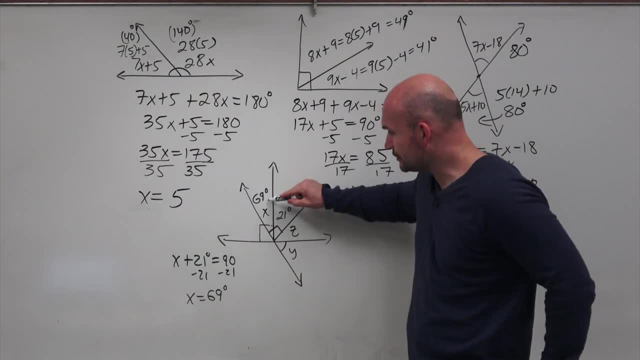 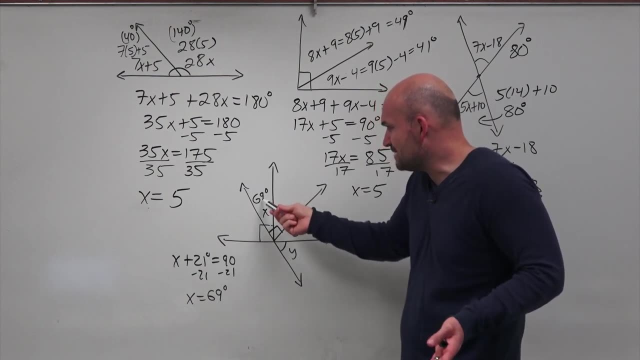 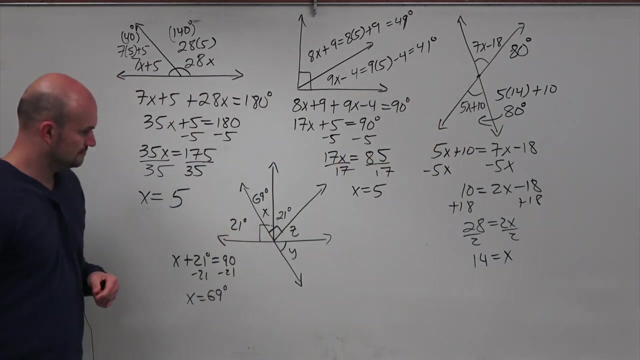 Now, another thing I recognize is 69 degrees, and this angle, whatever this angle is- is also going to be complementary, right? And so, obviously, if 69 and 21 are complementary, then 69, this has to be 21 degrees as well. OK, So now I want you to look at something. 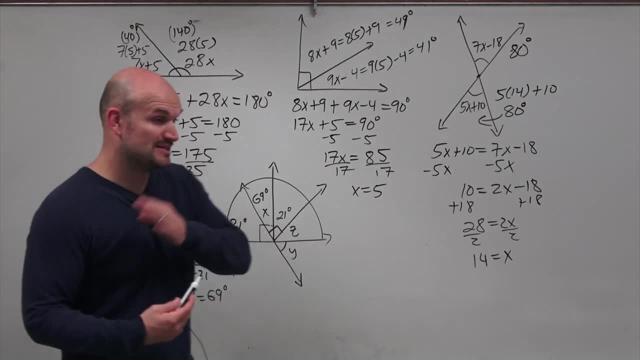 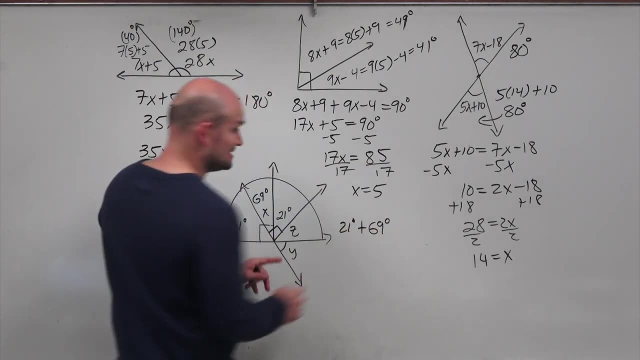 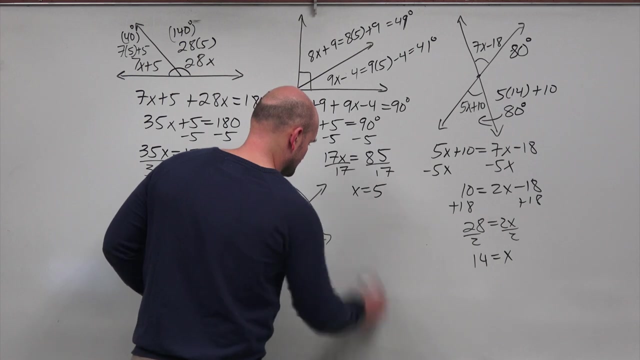 Now, if you look at this, I have this line right. So that means all of these angles are going to add up to 180 degrees. So right now I have 21 degrees plus 69 degrees, plus 21 degrees again, plus z- Uh-oh, I'm running out of space. So I have 21 degrees plus 69 degrees, plus 21 degrees. 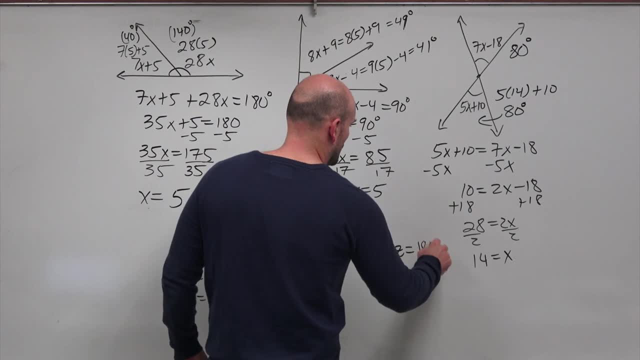 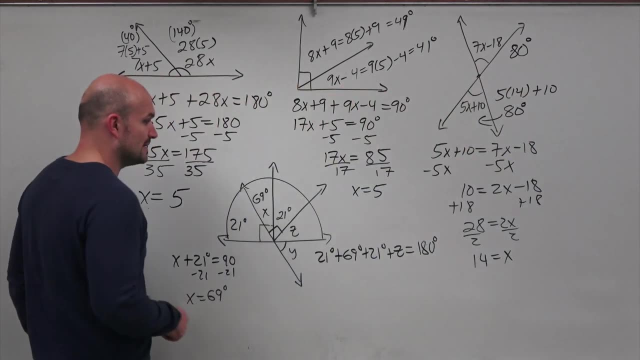 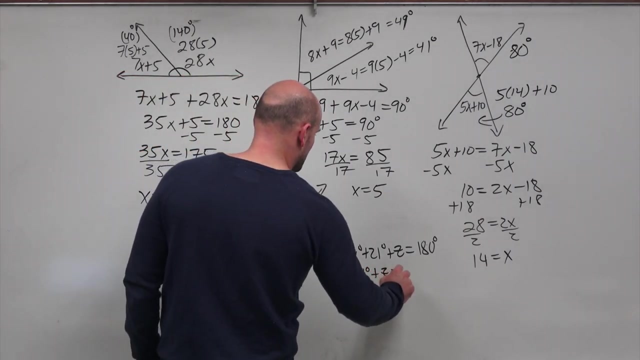 plus z is equal to 180 degrees. all right, Now we can go ahead and solve for my z. So when I go ahead and do that, let's see That's going to give me a 42.. That's going to give me 111 degrees plus z equals 180 degrees. 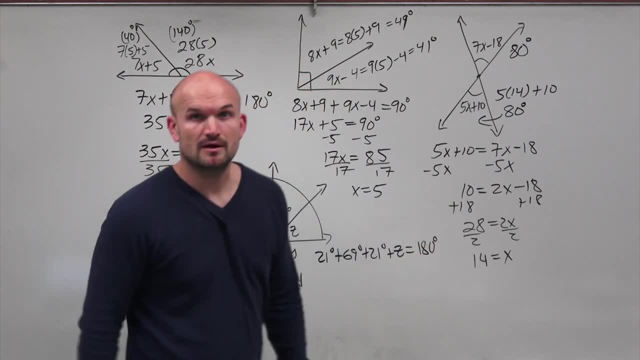 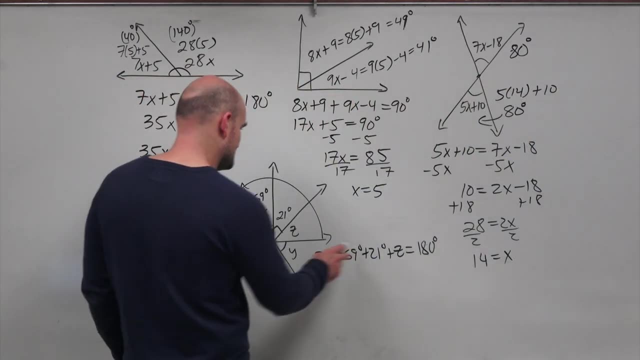 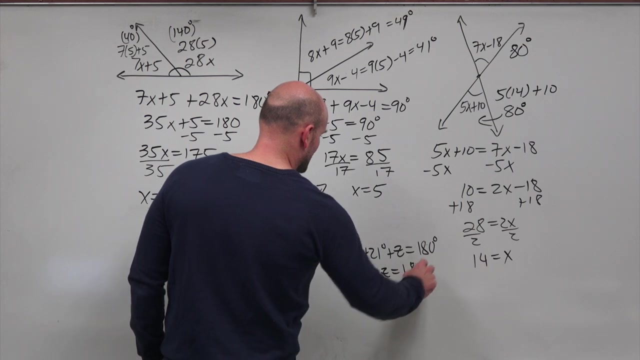 is equal to 180 degrees. all right, So now we can go ahead and solve for my z. So when I go ahead and do that, let's see that's going to give me a 42.. That's going to give me 111 degrees plus z equals 180 degrees. 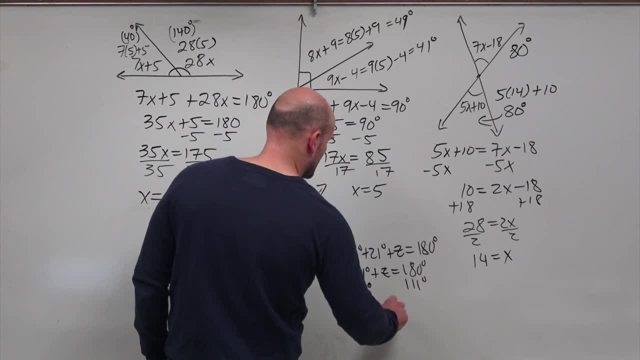 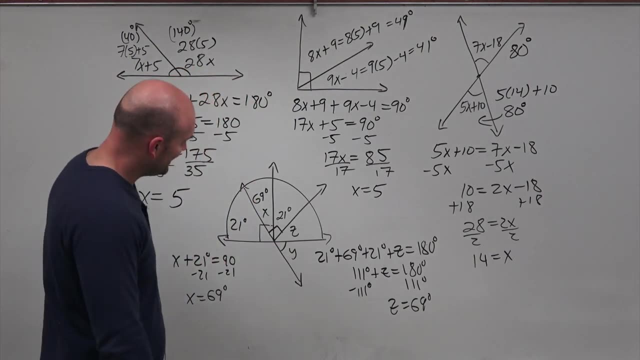 When you subtract 111 degrees you get z equals 69 degrees. Very, very interesting. And then the last relationship I can see is: you can, hopefully you can recognize here that I have some vertical lines here I have. these two lines are vertical. 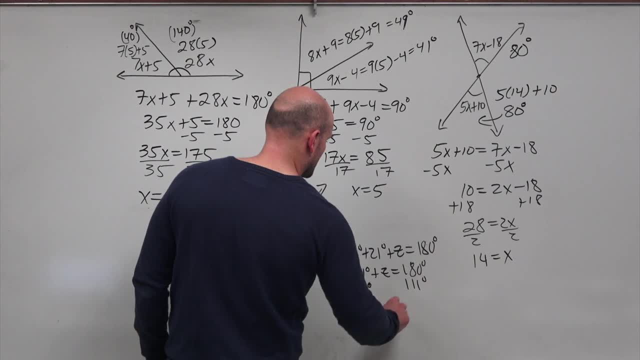 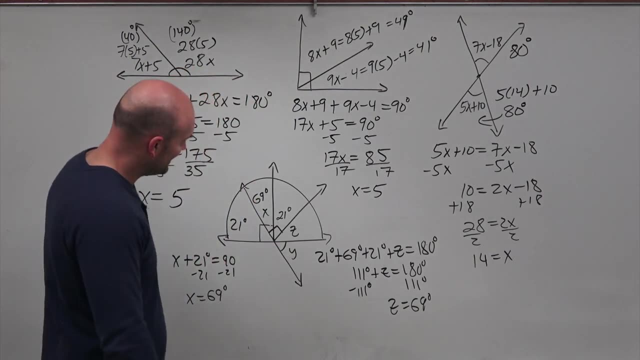 When you subtract 111 degrees, you get z equals 69 degrees. Very, very interesting. And then the last relationship I can see is: hopefully you can recognize here that I have some vertical lines here. I have these two lines here. I have these two lines here. 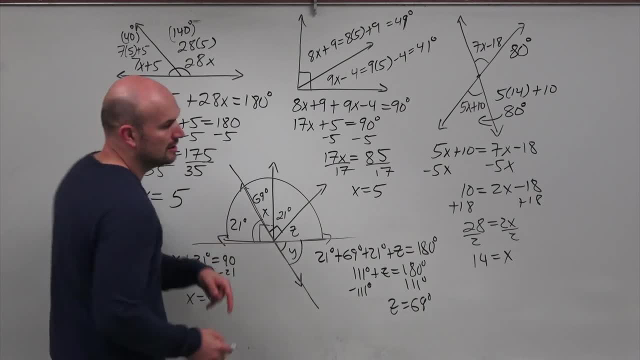 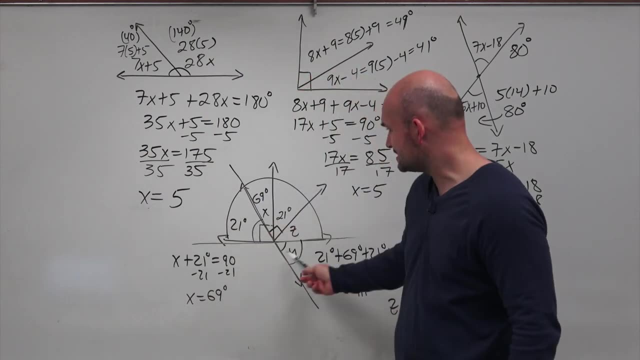 I have these two lines here. These two lines are vertical. That means they are creating their vertical lines. They're intersecting lines, so they're creating vertical angles. So if this angle is 21 degrees, then that angle also has to be 21 degrees. 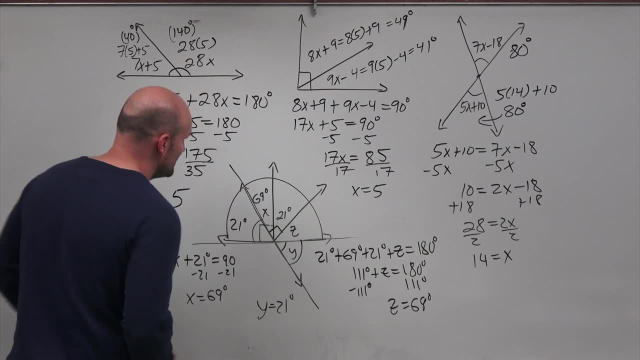 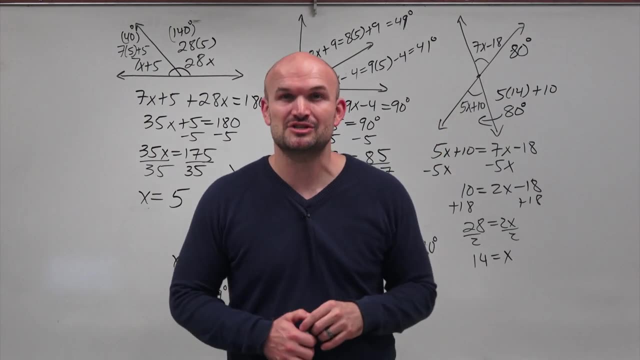 So, therefore, I can say y is equal to 21 degrees. So there you go, ladies and gentlemen. That is how we use complementary, supplementary as well as vertical angles to find the missing measures of an angle. Hope to see you on the next example and plenty more examples in my playlist. Cheers.